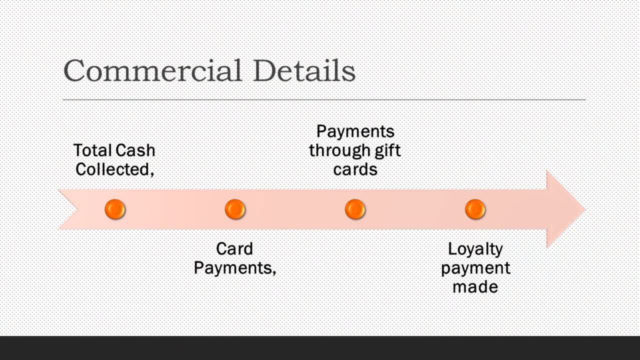 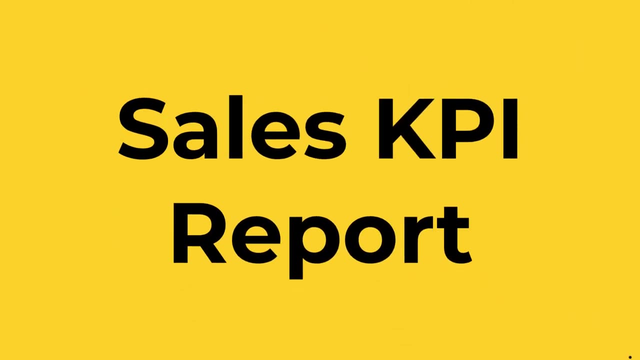 selling for all the departments. This report also contains all the commercial aspects of the store, such as total cash collected, card payments made, payments made through gift cards and loyalty payments. All these things are covered in detail in the store manager recap report. The third report is called as sales KPI report. 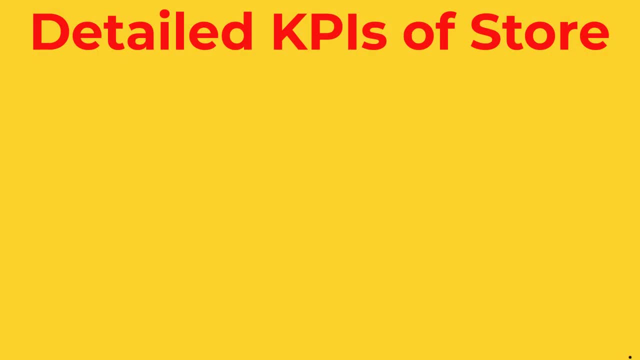 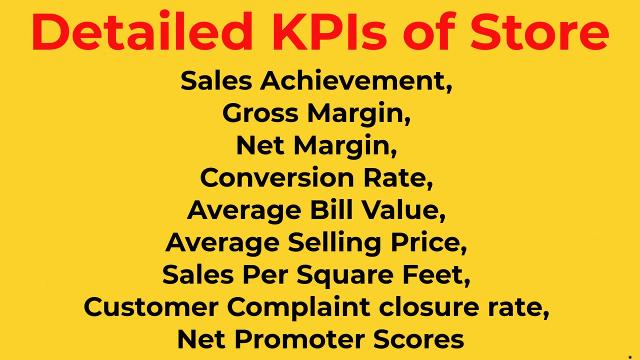 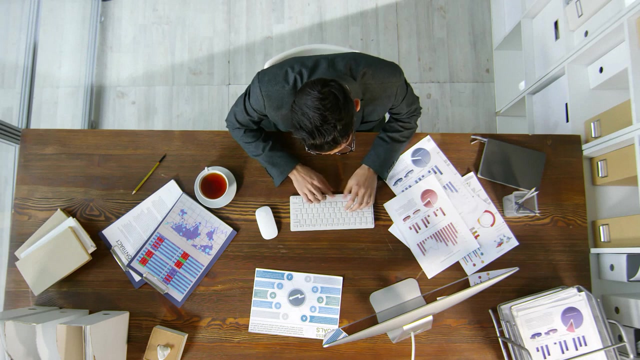 This report has a detailed analysis of all the KPIs of the store, which are: sales achievement, gross margin, net margin conversion rate, average bill value, sales per square feet, customer complaint closure rate and net promoter scores. With the help of this report, one can analyse how well the store is performing and also 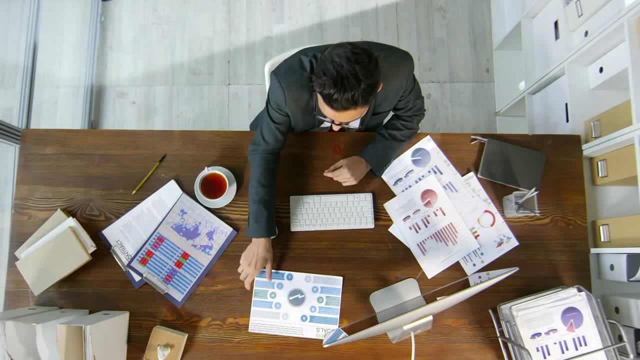 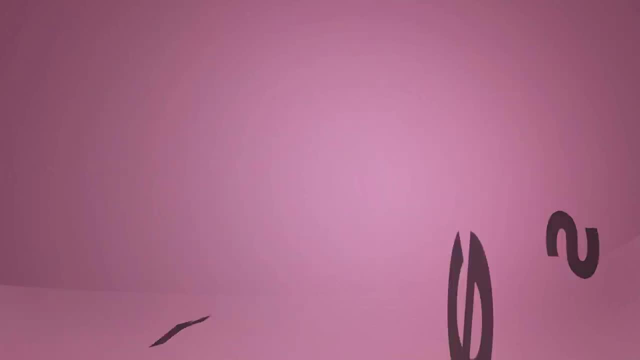 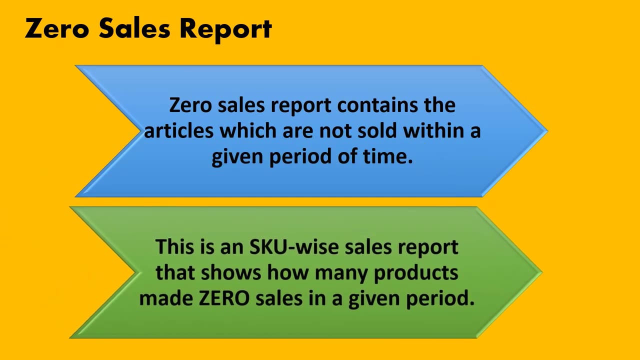 one can analyse this report to make sure all the parameters are improved and the KPIs are taken care of. As the name suggests, zero sales report contains all the articles which are not sold within a given period of time. This is an SKUI sales report that will show how many products made a zero sales within. 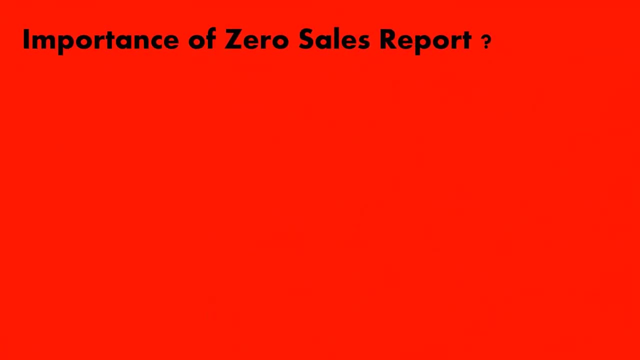 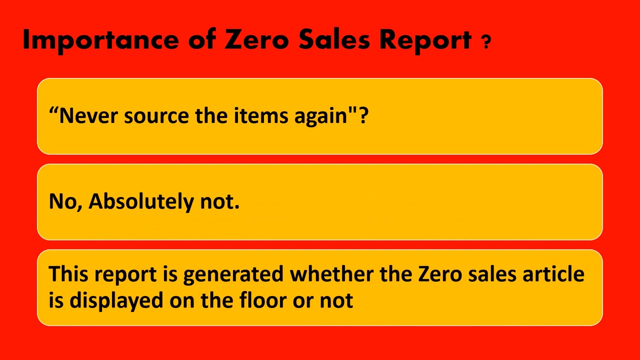 a given period of time. So what is the importance of zero sales report? Is this report generated to never source the items again? No, absolutely not. This report is generated to check whether the zero sales article is displayed on the floor or not. Most of the time, the zero sales article will be displayed on the floor. 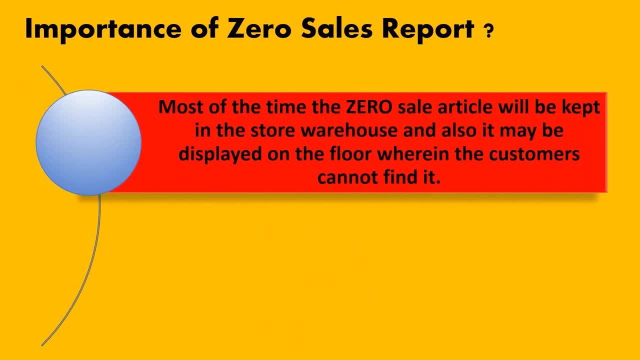 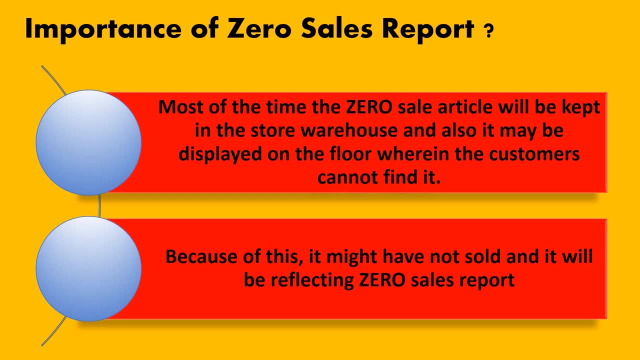 Most of the time the zero sales article will be displayed on the floor. Most often the sales article will be kept in the store warehouse and also it may be displayed on the floor where in the customers cannot find it. Because of this, it might have not sold and it will be reflecting in zero sales report. 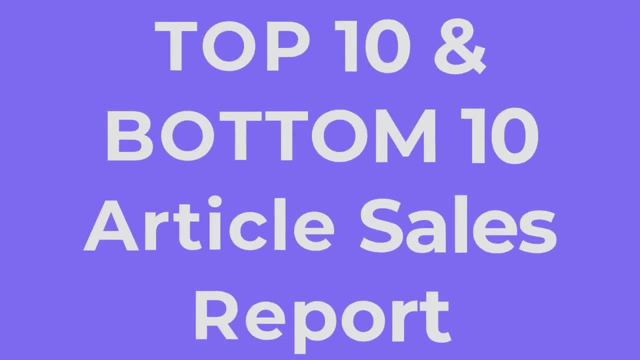 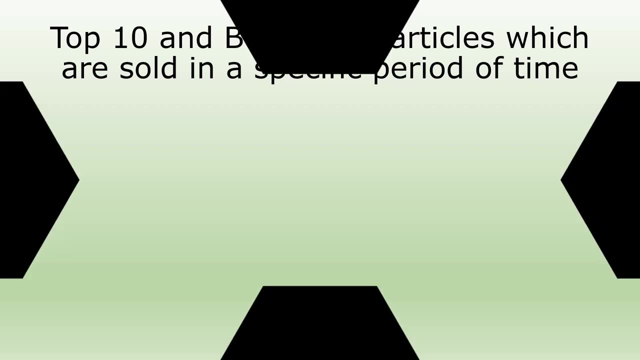 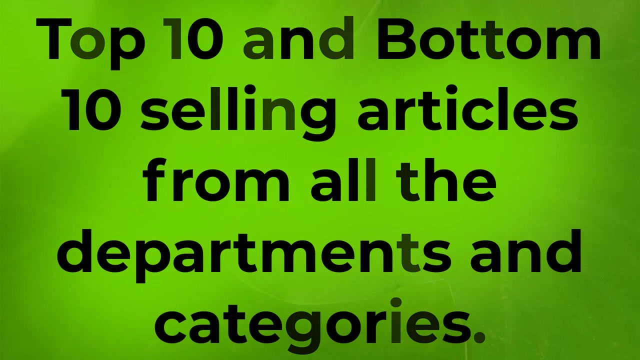 5. So this report contains the top 10 and bottom 10 articles which are sold during a specific period of time. This is Department and category wise sales reports. This report will contain top 10 and bottom 10 selling articles from all the departments. 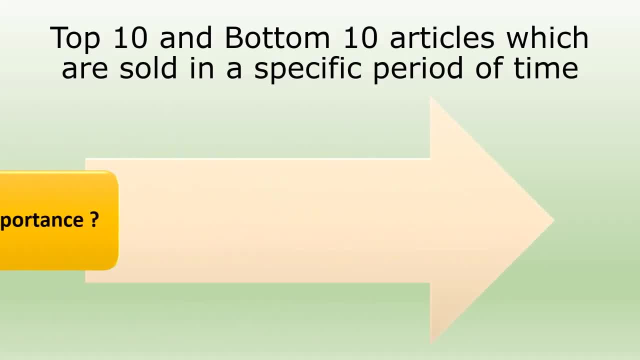 the respective categories. So what is the importance of this report? This report will help in planning the inventory. One must make sure that we have sufficient stocks of top selling articles so that those will not be stock outs. Also, we must check whether we have sufficient. 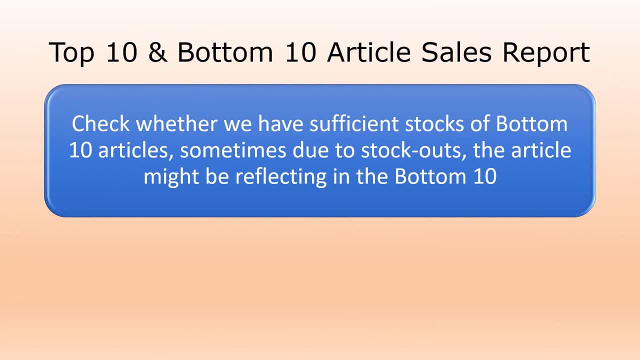 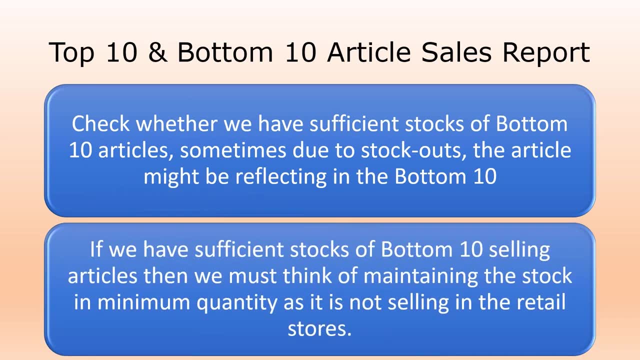 stocks of bottom 10 articles. Sometimes, due to stock outs, the article might be reflecting in the bottom 10.. If we have sufficient stocks of the bottom 10 selling articles in the store, then we must think of maintaining the stock in the minimum quantity, as it is not selling in the 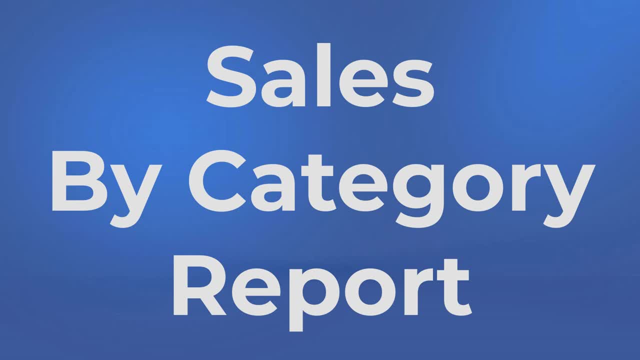 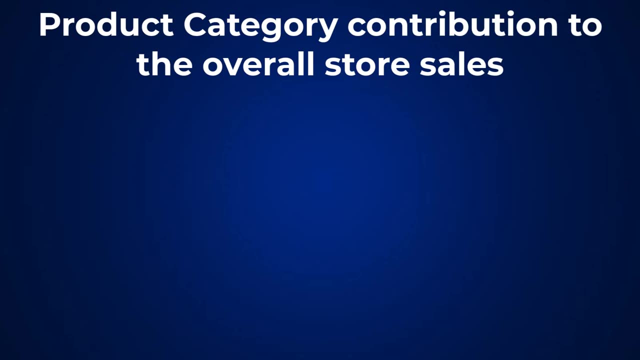 retail store. The sixth report is called as sales by category report. This report will help us to understand how much sale a particular product category is contributing to the overall store sales. This report can be generated on the department level as well as the product category. 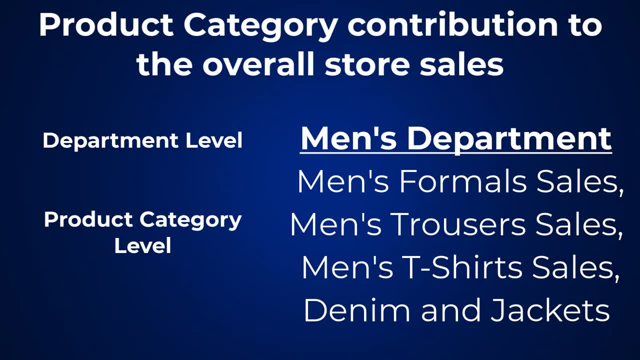 level. For example, you can generate reports of men's department as a whole and also men's formal sales, men's trousers sales, t-shirt sales, denim and jacket sales, so on and so forth. Similarly, it can be done for the women's wear and 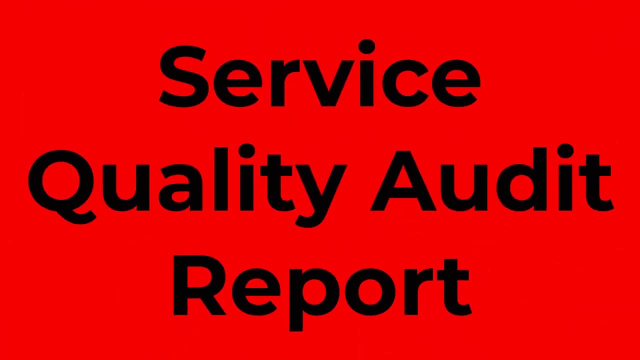 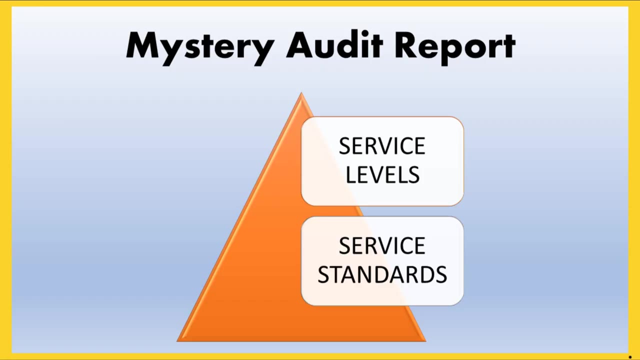 kids wear category also. So the seventh report is called as service quality audit report. Service quality audit report is also called as mystery audit report and it will tell the service level and the service standards of the given retail store. The mystery audit happens once in every. 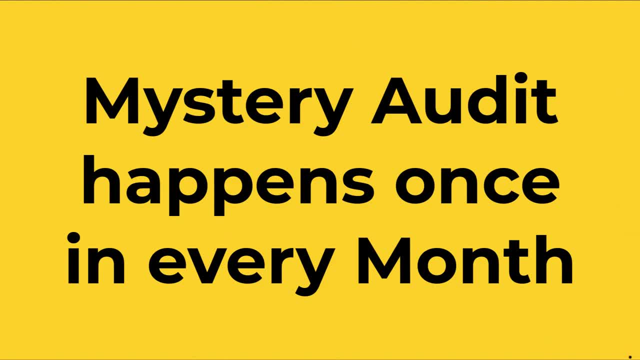 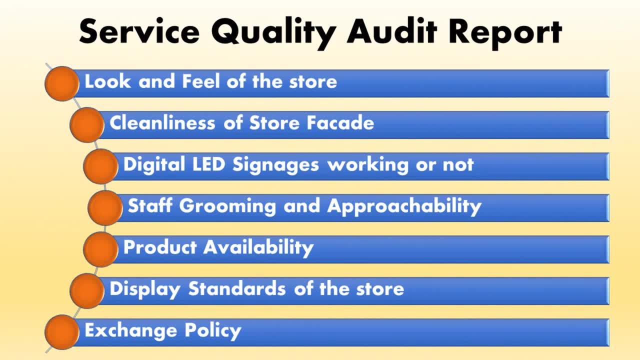 month and the auditor will judge the store on the following parameters, which are: look and feel of the store, cleanliness of the store facade. digital led signage is working or not in the store. what is the staff grooming and what are the approachability, the product availability in the 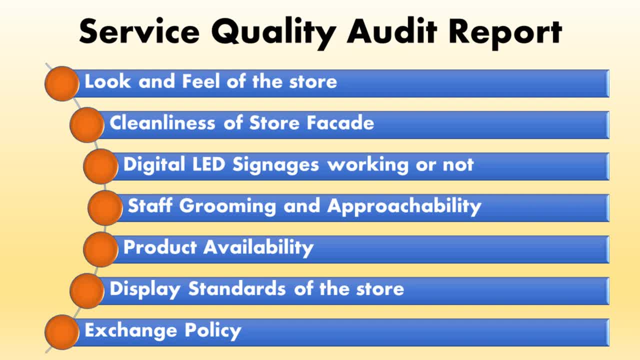 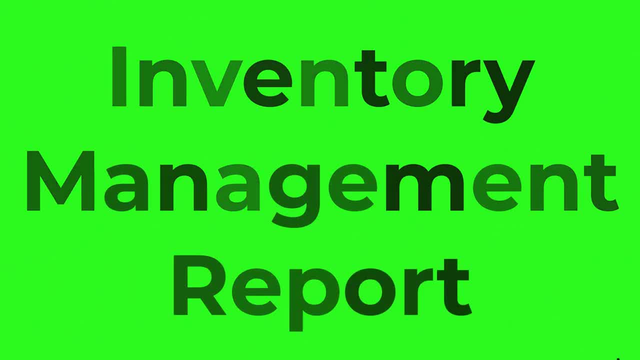 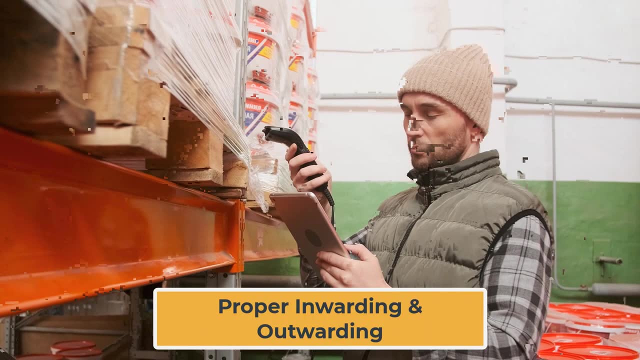 store. display of the product availability. display of the product availability in the store. display of the product availability in the store. display of the product availability. and what are the performance of the product? So all of these parameters are evaluated by the mystery auditor. 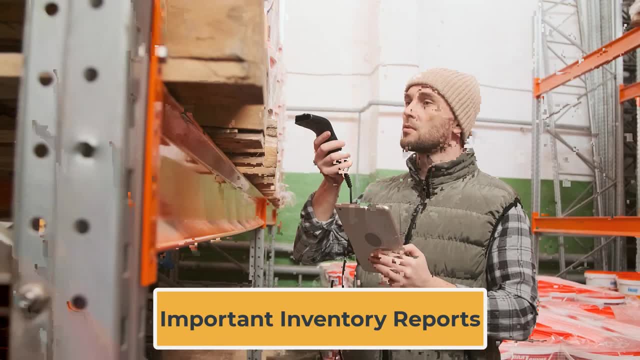 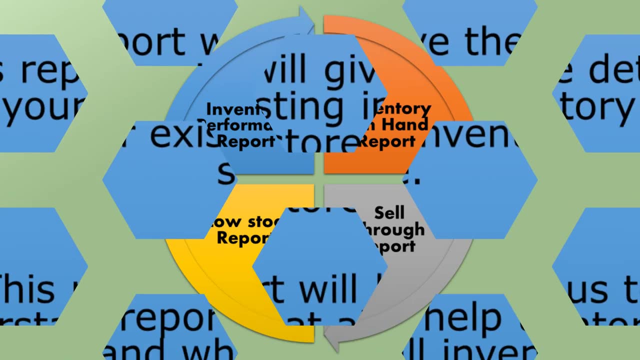 Now coming to the eighth kind of reports, which are inventory management reports. Inventory management involves proper maintenance of stock, inverting and outwording as per the SOP and maintaining overall healthy inventory. To track this, we have some of the important inventory reports report. the report will give the details about your existing inventory in the store. 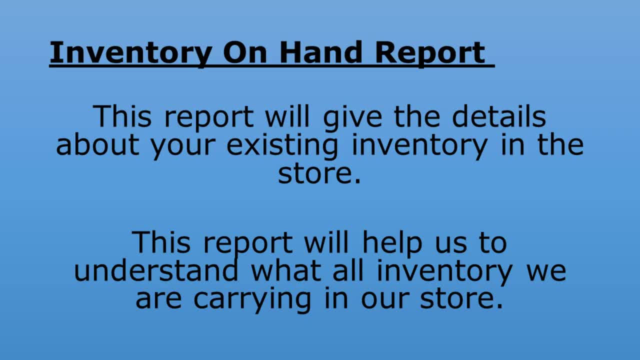 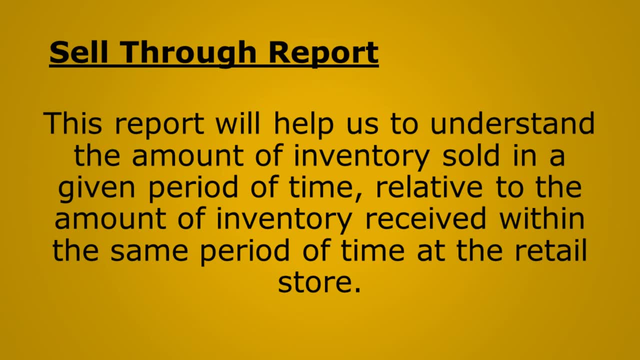 This report will help us to understand what all inventory we are carrying in the store. So the next report is sell-through report. This report will help us in understanding the amount of inventory sold in a given period of time relative to the amount of inventory received within the same period of time. 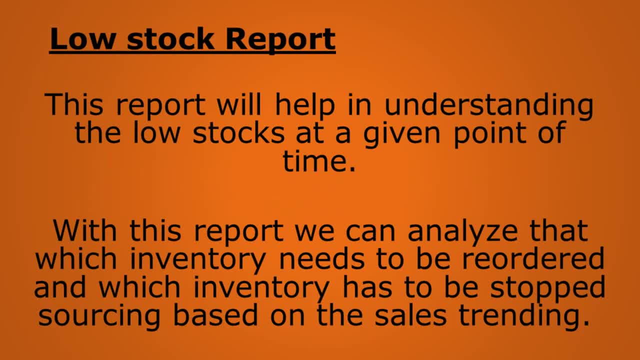 The next inventory report is called as low stock report. This report will help us in understanding the low stocks at the given point of time. With this report, we can analyse that which inventory needs to be re-ordered and which inventory has to be stopped sourcing based on the sales trending.